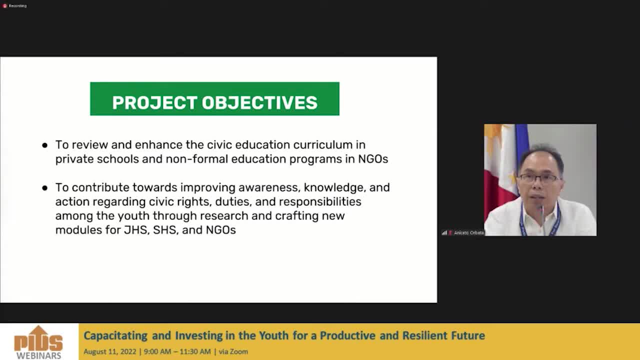 The University of the Philippines is the one examining the curriculum modules of the public schools. Of course, the private schools are also following the standards set by the Department of Education, but they have more leeway in terms of introducing curriculum modules for private schools in the public schools. So they have more leeway in terms of introducing curriculum modules for private schools in the public schools, And so they are more likely to use the curriculum and the UNHCR as a tool to support the career of the private schools and non-governmental organizations. 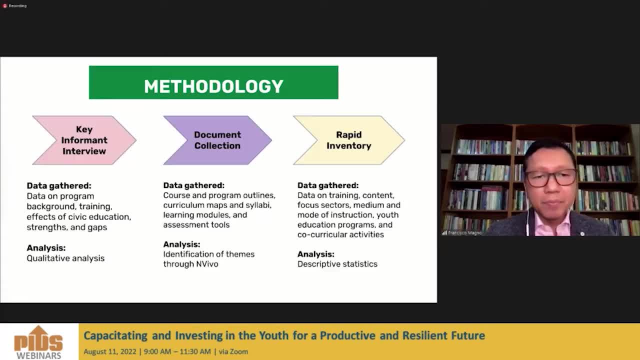 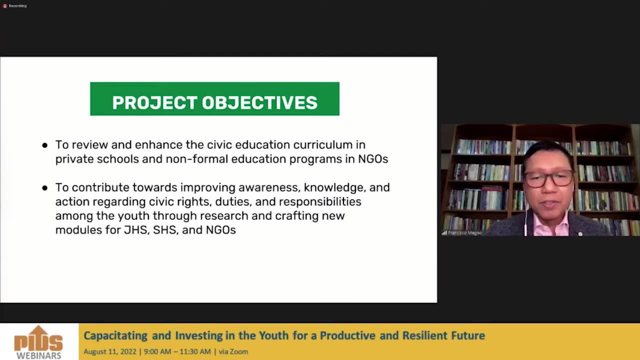 so that they can improve their organizations and their efforts to achieve the educational prestige and the UNHCR as a tool to support the educational prestige of private schools and non-governmental organizations. The second key objective is to contribute towards enhancing or improving awareness, knowledge and action regarding civic rights, duties and responsibilities among the youth. 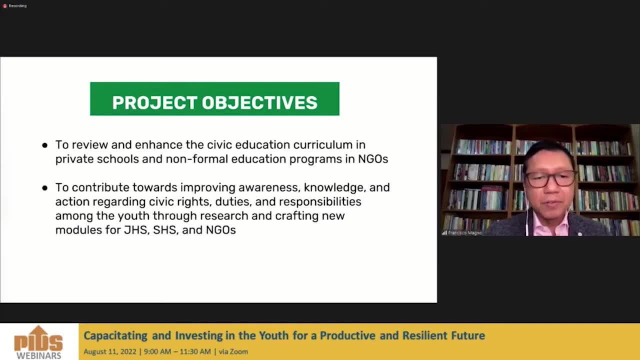 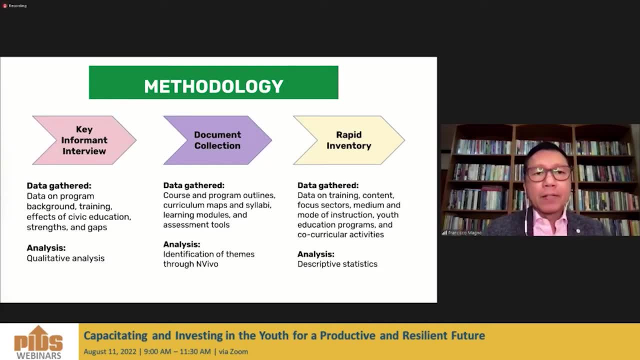 to research and crafting new modules for junior high school, senior high school and NGOs. So this is the methodology. So I'm presenting to you the research results, the preliminary results that will inform module development And these are the methods We conducted key informant interviews. 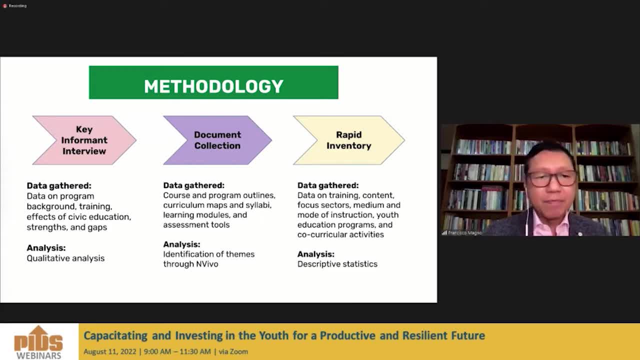 We conducted document collection and rapid inventory. We gathered data on a program, a book, program, background training, effects of civic education, strengths and gaps. These are from the insights shared by our key informant interviews, So they include the administrators of private schools, NGO leaders and also coordinators. 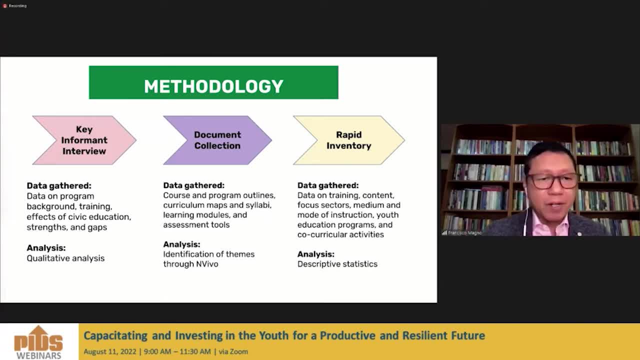 of the junior and senior high school programs. So, in terms of documents collected, we gathered a course and program outlines, curriculum maps and syllabi, learning modules and assessment tools. The rapid inventory consisted of asking for data on training content, focus sectors. 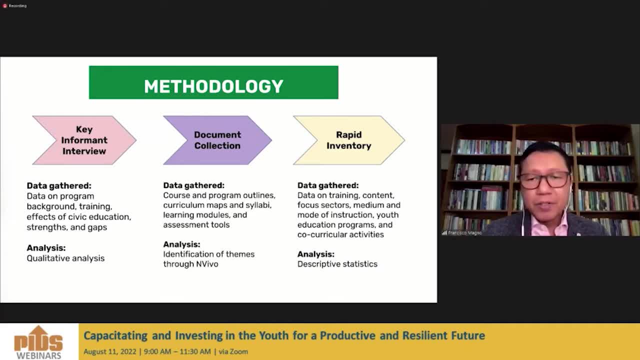 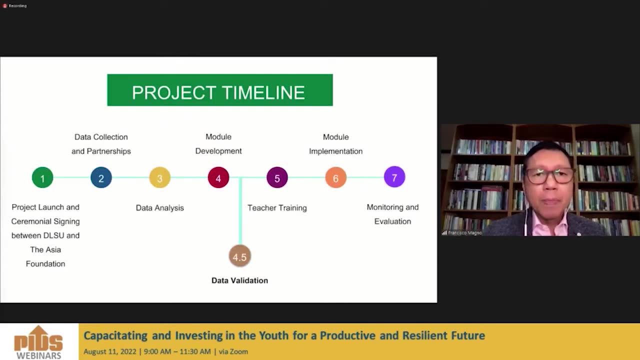 medium and mode of instruction: youth education programs and co-curricular activities. So we use in vivo software. in terms of the qualitative content analysis, Next slide. So just to provide you with the project timeline. So we've been doing this project for the past. 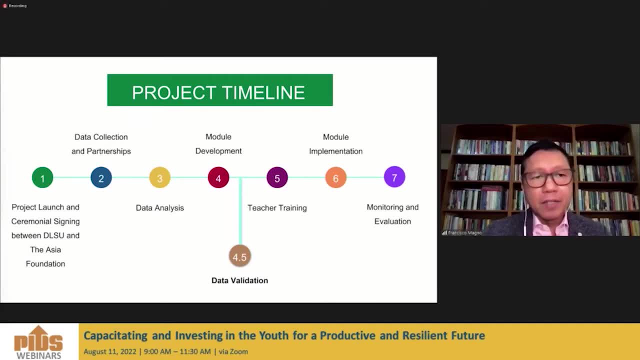 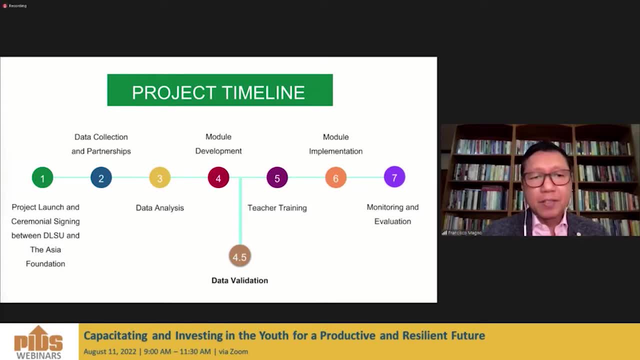 the PEYAK, or the Philippine Educational Assistance Committee, and the PACU, or the Private Association of Colleges and Universities. We've also been developing partnerships with individual high, individual high educational institutions that offer senior high school, including Bicol University. So 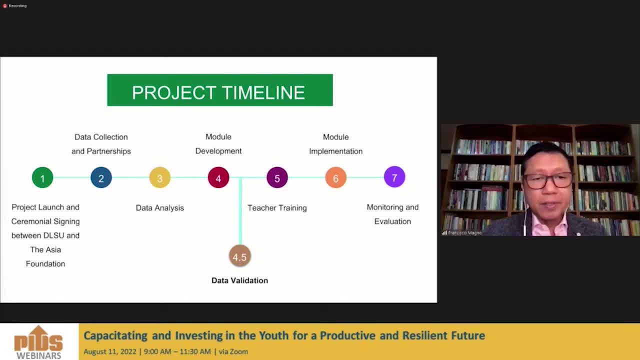 individual high educational institutions that offer senior high school, including Bicol University. So we actually inked that partnership with Bicol University And so we conducted this preliminary analysis that I will share with you this morning, and our module and curriculum specialist, Lea Castillo, who is from De La Salle. 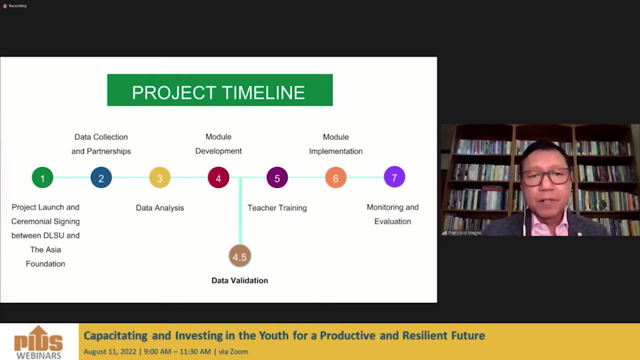 and our module and curriculum specialist, Lea Castillo, who is from De La Salle, Sal, Santiago-Sabel, developed a draft module. In fact, she developed three modules: one for junior high school, for senior high school and NGOs. So we'll also be doing. 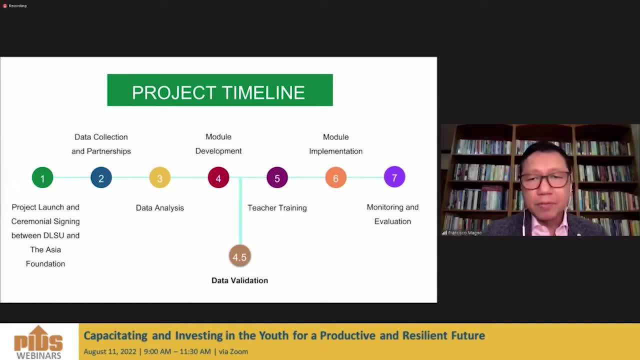 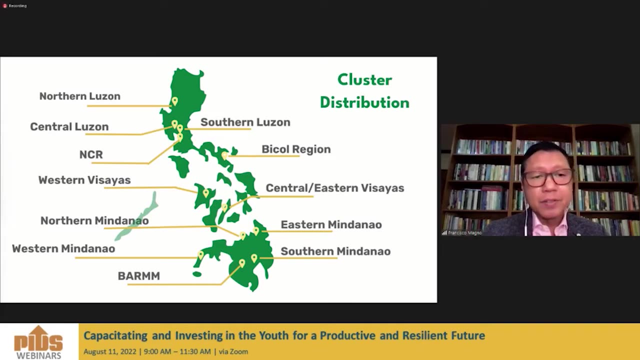 teacher training. We had a data validation activity last week and we will proceed with module implementation and monitoring and evaluation. Next slide. So this is the coverage in terms of the regions. So I mentioned rapid inventory, So we went to different regions. Of course we were hampered by protocols, health protocols. 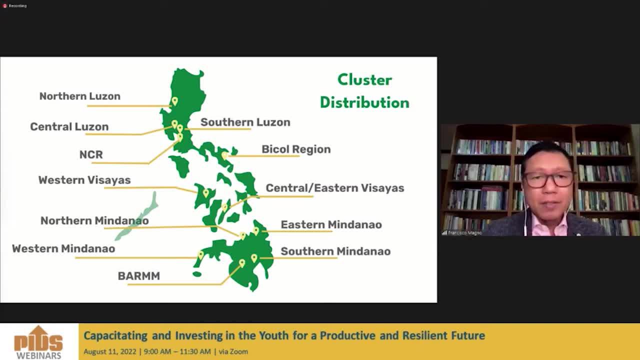 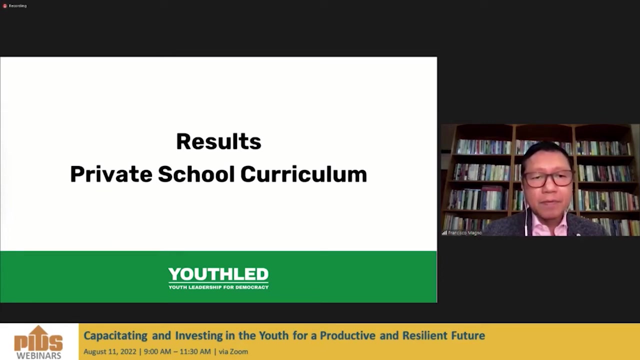 so we conducted it through Zoom, And so these are the regions that we covered. We had more than 100 partner institutions, including private schools and NGOs. Next slide: Let me now show you the results of our examination of the private school curriculum. Next slide. 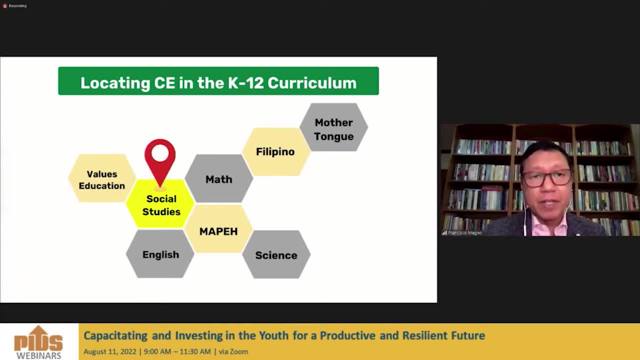 So social studies within the ecosystem of civic education in the K to 12 curriculum is primarily located in the social studies learning domain, although it does not preclude the inclusion of civic education in the other subjects. So this is something that we are actually discussing. 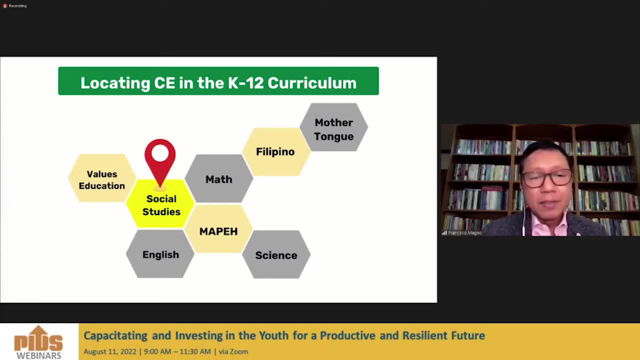 Like some of the examples perhaps in mathematics, can include content from the social studies as well as the observational context, which is a very popular topic for social studies. So we can also include some of the content from the social studies as well as the observation and evaluation, as well as the evaluation period, The first slide. 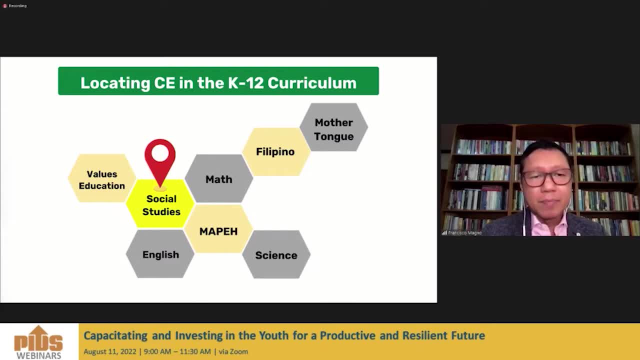 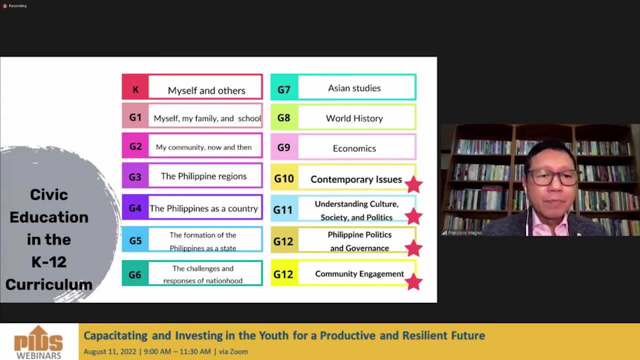 the other learning areas. But what we found out? that primarily social studies is the key subject area where civic education is incorporated. Next slide: So if you take a look at the different grade levels from K to 12, there is content that is available at the various grade levels. 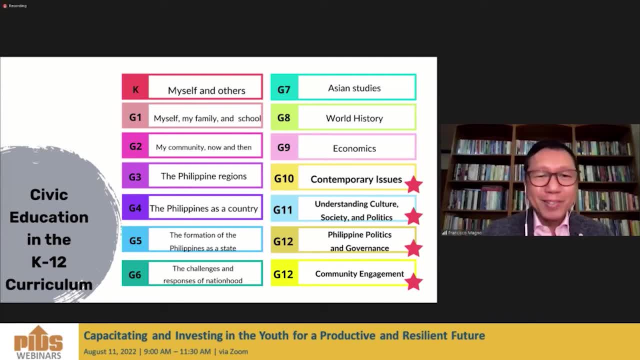 So for me this is very interesting, since I, of course, I went to, I got my basic education a long time ago, and look at the, the titles of these civic education areas, For in kinder you have myself andush others. So it's a learning period where the individual, the individual Filipino, is learning. 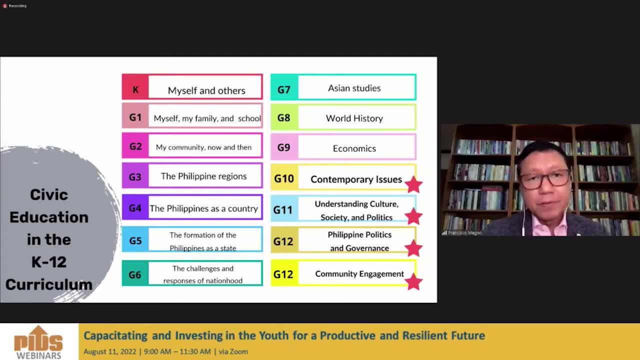 to connect himself or herself with others, So he or she is not alone in this world. in terms of exercising rights as well as performing responsibilities. So grade one: myself, my school and family, So the sphere of relationship is growing. And in grade two, 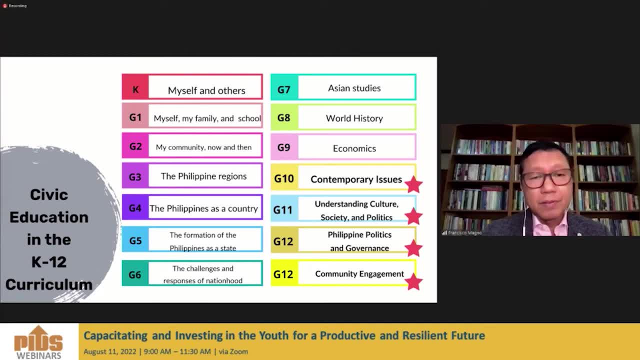 you really have a broader sense. Of course that's the competence or competency that is pursued: my community now and then. So it's even a sense of history of the local community. In grade three you have now a concept of a region. 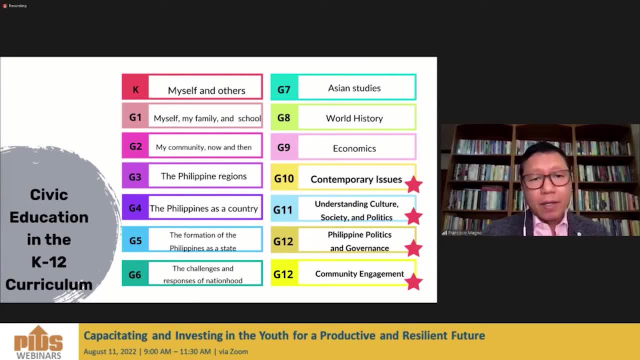 Belonging to a region, the Philippine regions. Understanding the different Philippine regions, of course, Grade four, the Philippines as a country. So you now begin to have a sense of being part of a country and a nation. So there is a cultural sense there of identity. 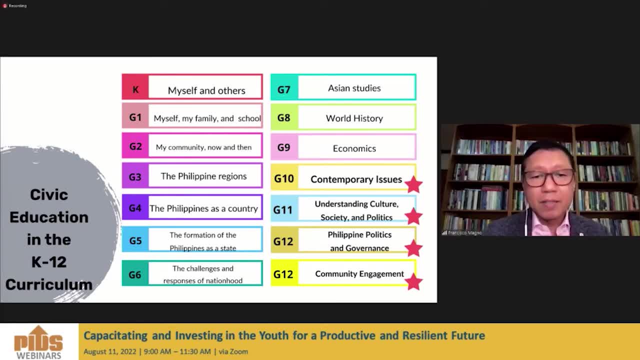 In grade five, the formation of the Philippines as a state. So you belong now to a political community. So you are now Developing this concept of a citizen belonging to a state and a state as part of a bigger community. And now you begin in grade six to connect the state with the nation. So the state 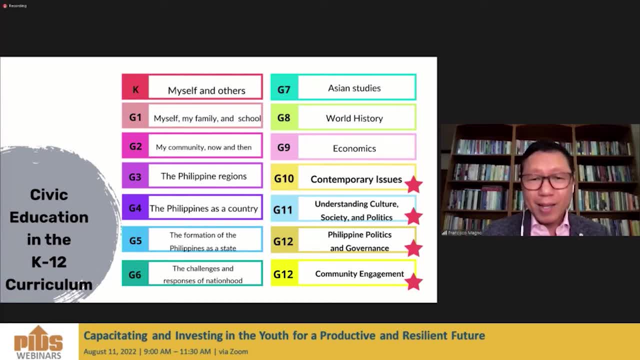 as a political entity that collects taxes and that formulates and implements laws and policies. But then you are part of a cultural entity, So you have a political entity called the nation. So that, therefore, the formation of concept of a nation state and then the nation state, 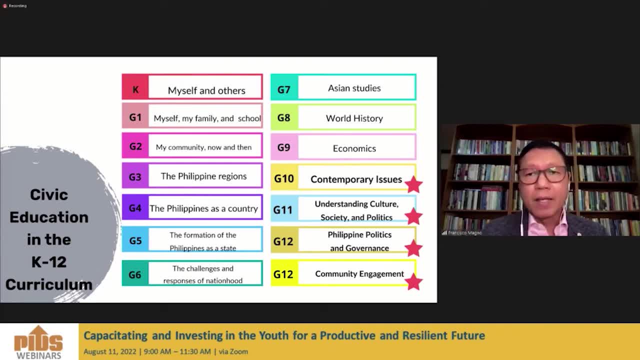 the Philippine nation state is part of Asia and Southeast Asia. Grade seven: Asian Studies. and Asia belongs to the world or is part of the world. So the developments of our countries part of world history. and grade nine: Of course we understand the globe. 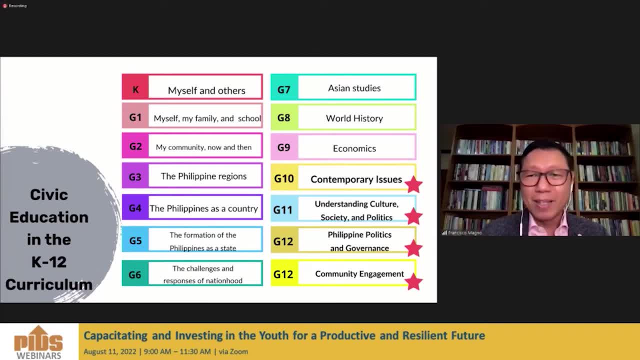 We understand the climate, globalization, and we should understand economics, market development. and so, with grade 10, you all have these notions of identity, whether political, cultural, economic. you belong to a country, to a state, you are a citizen of the world and the earth. and so, in grade 10, 11 and 12, you begin to 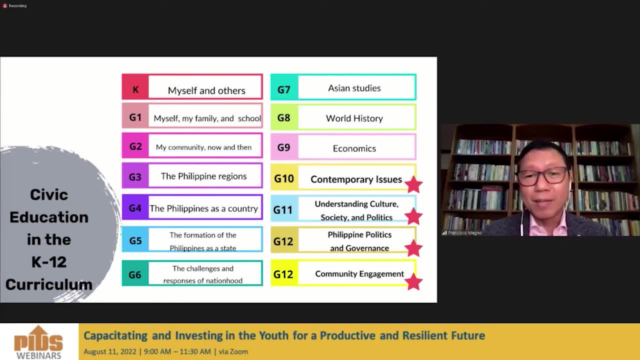 bring together all these concepts and use these concepts in understanding contemporary issues. grade 11: understanding culture, society and politics, so those different sense of identity. you begin to bring it together in a way that you can develop insights and you can analyze what's happening around you. in grade 12: 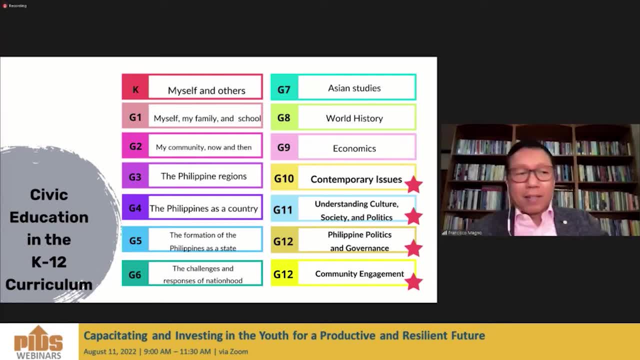 12 philippine politics and governance, and i suppose in grade 12 you are. you, you're probably turning 18 and you can now vote. it depends, of course, on the electoral cycle and grade 12 community engagement next slide. so civic education in junior high school. 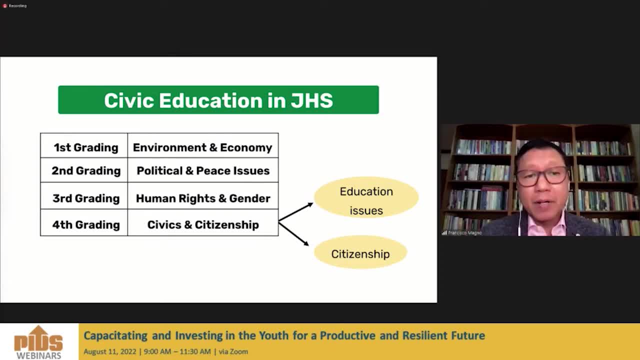 especially in contemporary issues. so we can divide it into four grade levels, uh grade phases or periods, rating grading periods. in the first grading you have environment and economy as content. second grading, political and peace issues. third grading, human rights and gender. and fourth grading, civics and citizenship. usually in civics, 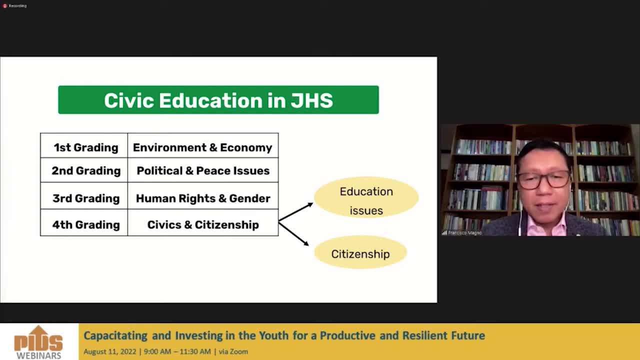 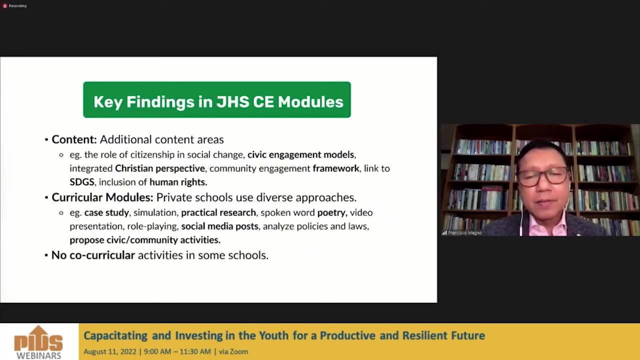 and citizenship. we found out that what are tackled there is a combination of education issues and citizenship issues. next slide in looking at the different civic education modules used in private junior high schools. as i mentioned, private schools have more space in terms of introducing additional content areas. these are the things that we found out. the focus: some of the focus areas are the role of citizens. 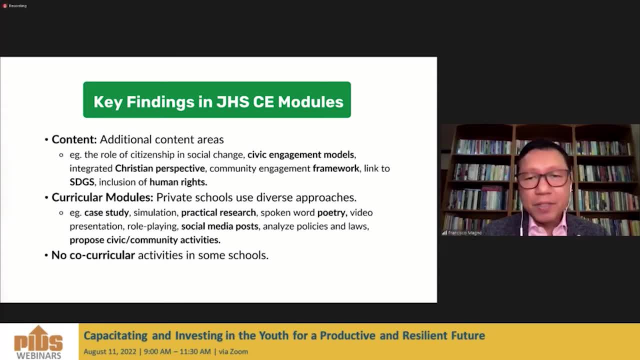 and the level of Santi. we always say that more rules are needed in the school environment. the introduction of civic engagement models, the integration of christian perspectives- as we know, private schools have our have christian affiliations and community engagement framework is goals- and the inclusion of human rights In terms of the curricular modules. 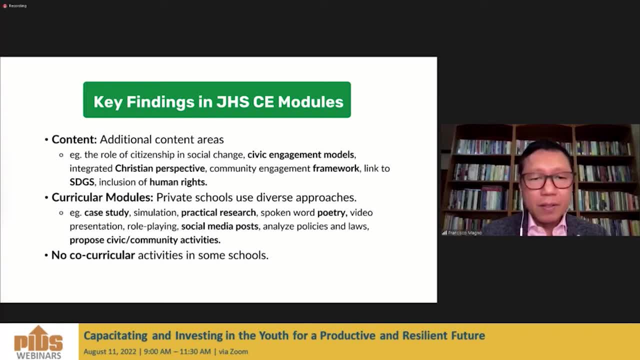 private schools use diverse approaches, including case studies, simulation, practical research, poetry, video presentation, role-playing, social media posts, analysis of policies and laws and proposing civic and community activities. However, there are some schools that do not have co-curricular activities. Next slide: 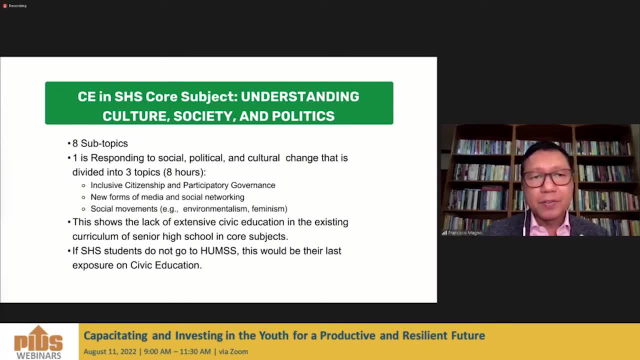 Okay, civic education in the senior high school core subject, which is understanding culture, society and politics. This subject has eight sub-topics. One responds to social, political and cultural change. that is divided into eight topics and that amounts to eight R's. 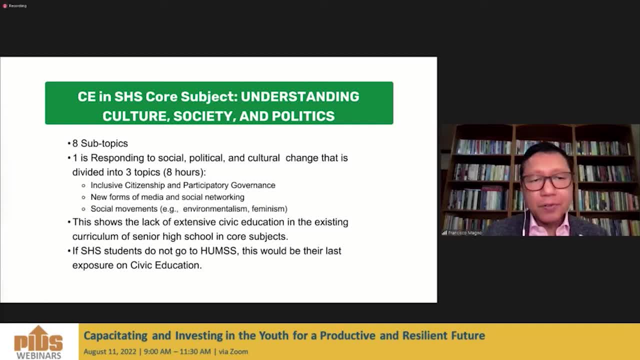 The topic that are included are inclusive citizenship and participatory governance, new forms of social media and social networking, social movements, including environmentalism and feminism. This result indicates the lack of extensive civic education in the existing curriculum of senior high school in core and other sub-topics. As you notice, it's only eight R's, So apparently in the subject-area. 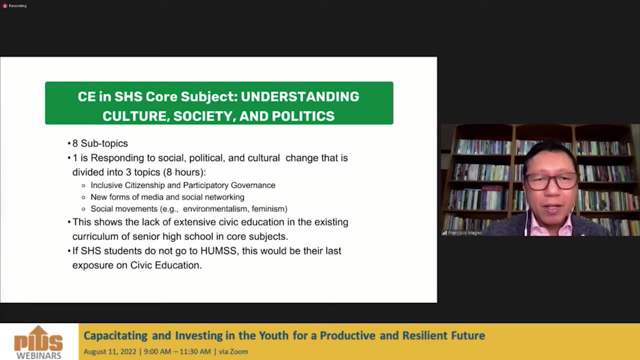 understanding culture, society and politics. there's more discussion of the culture and societal part rather than the political and citizenship part. Hence, if senior high school students do not go to YUMs their last exposure on civic education, because under HUMES there is the 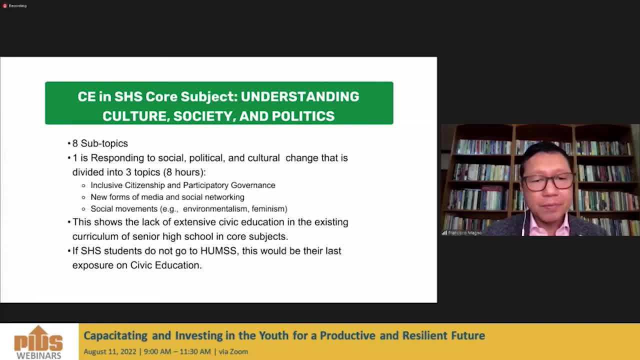 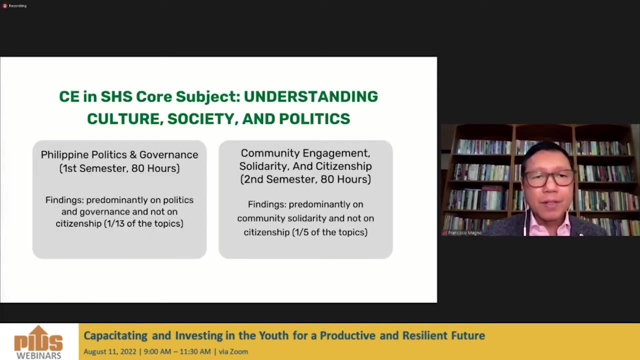 okay, we'll transition to the next slide. okay, let's look more closely at the division in terms of the number of hours in understanding culture, society and politics. so you have Philippine politics and governance first. this is taught in the first semester for ATRs, and community engagement, solidarity and 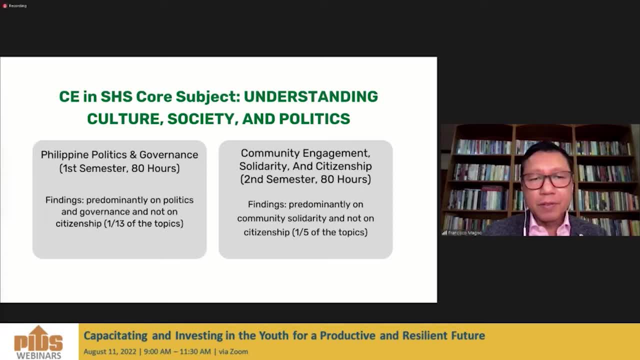 citizenship also ATRs for second semester. so we noted that in Philippine politics and governance the focus is on politics and governance and not enough on citizenship. so only 1- 13th of the topics are primarily citizenship and in the discussion on community engagement, solidarity and citizenship, it's predominantly on community solidarity and not 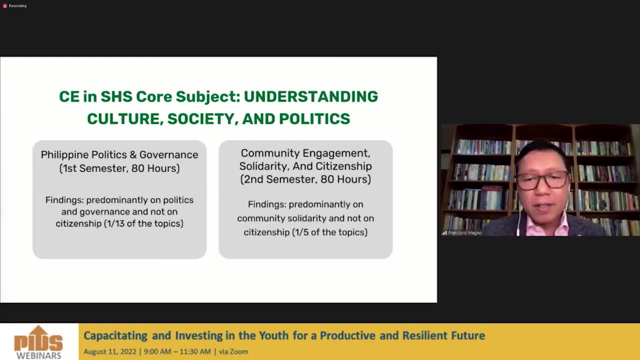 on citizenship. so apparently there is a need to introduce more content on the citizenship portion. so we may have to give attention to citizenship aspect because we always say, or there is always advocacy, let's have voters education prior to elections, during the campaign, vote wisely, but maybe it should be done prior to that in a continuous 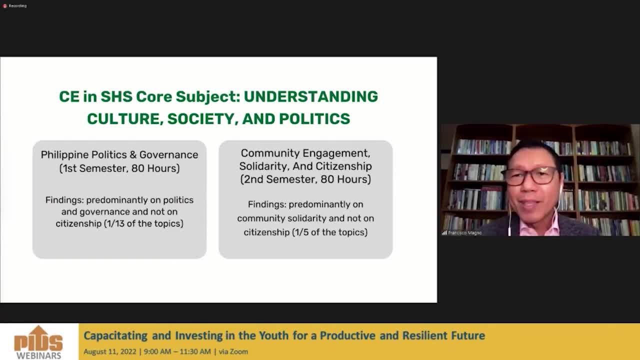 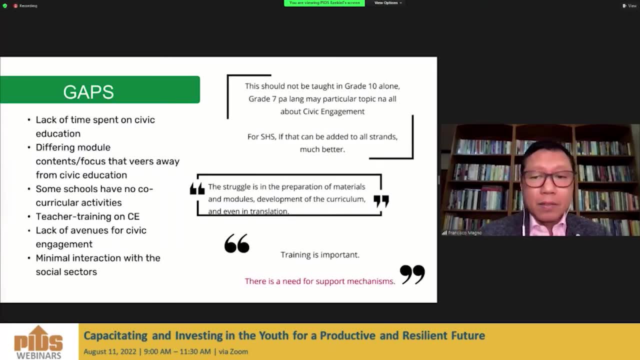 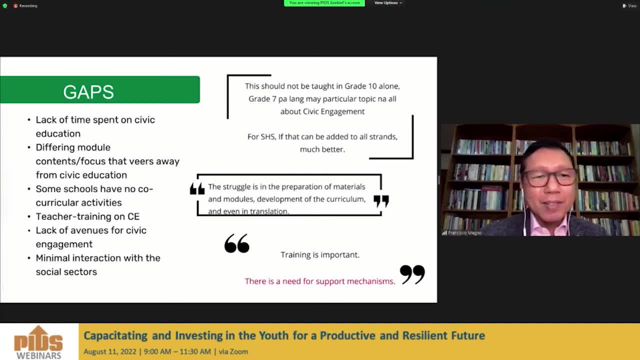 there is a lot of time spent on civic education. We use the NVivo content software to do this thematic analysis In terms of differing module contents. there are differing module contents and the focus veers away from civic education. Given this understanding, as I've been emphasizing, 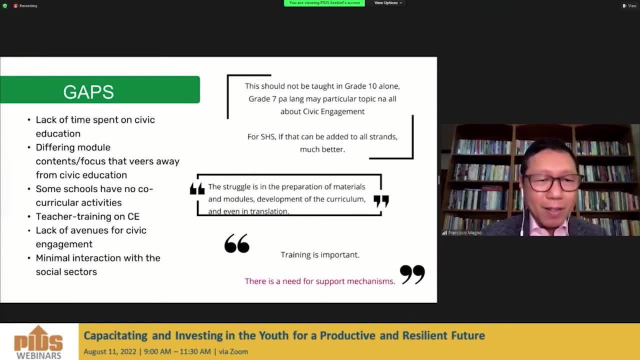 we need to bring back civic education. It's there in the curriculum but in the content area. Some schools have no co-curricular activities. There's a The need for teacher training on civic education. there is a lack of avenues for civic education or civic engagement and minimal interaction with the social sectors. 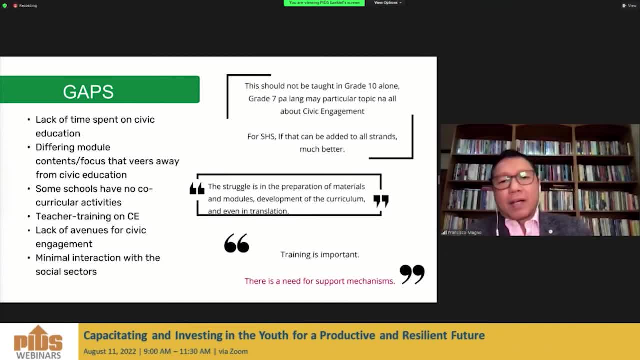 So eto mga direct quotes yung nasa kanan. One teacher said the struggle is in the preparation of materials and modules, development of the curriculum and even in translation. Teaching is important. There is a need for support mechanisms. Okay, on the right hand portion you can see a quote from one of our informants. this or: 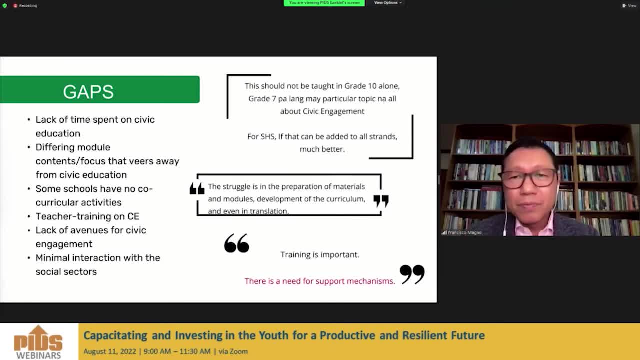 civic education should not be taught in grade 10 alone. Grade 7 pa lang may particular topic na about civic engagement For senior high school. it can be added to all strands and that would be much better. Okay, so good recommendations, especially because the K-12 program is being reviewed. 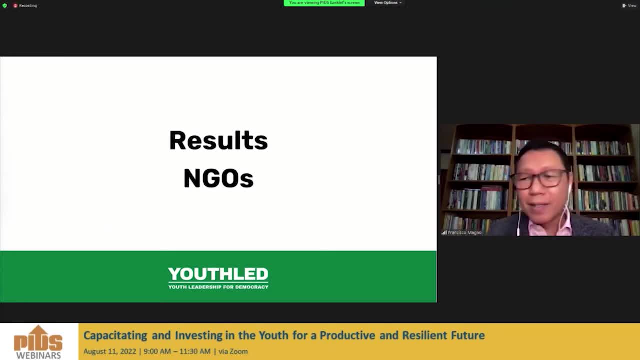 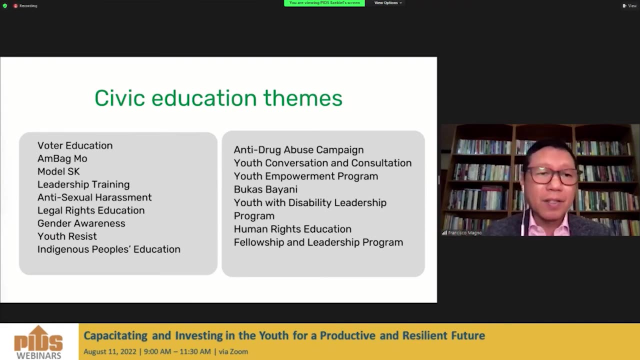 at this time. Next slide. Okay, I'll go quickly now. the results in terms of our research on NGOs. Next slide. So there's a variety of topics. So this is more of a non formal civic education, As you can see the variety of topics. 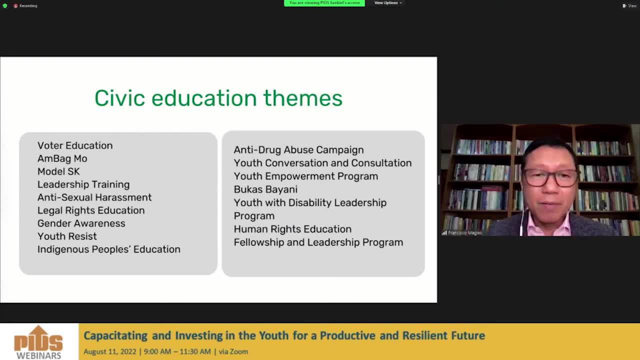 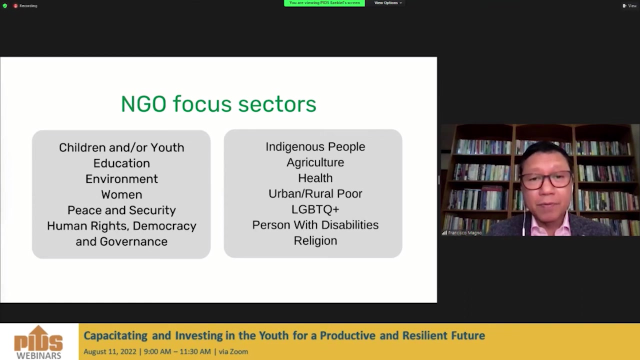 You can find Napanggit ko nga about their education. So it's being carried by NGO advocacy groups and anti-sexual harassment, youth empowerment programs, human rights education. Next slide In terms of the sectors, because NGOs, of course, are voluntary groups they work with. 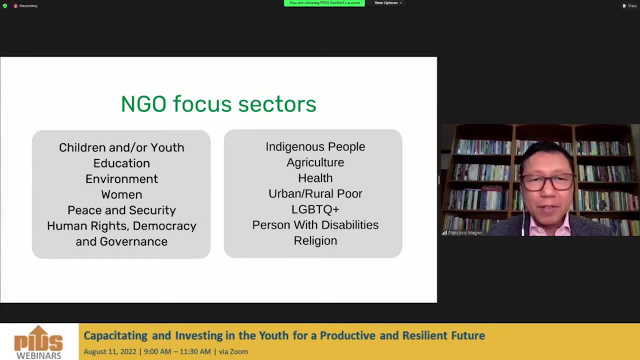 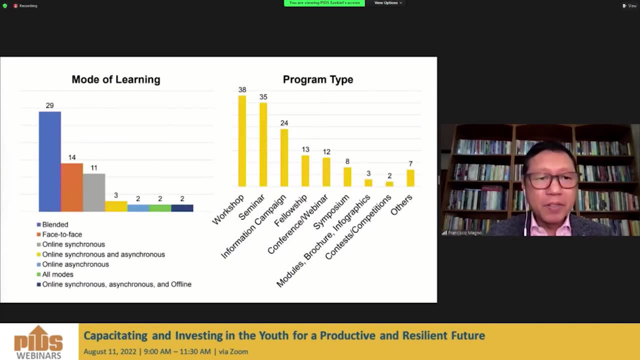 various sectors. You can see this Okay In terms of focus sectors. Next slide In terms of mode of learning, since we are in a pandemic, so you notice on the left side, blended learning is the key or the main mode of learning. 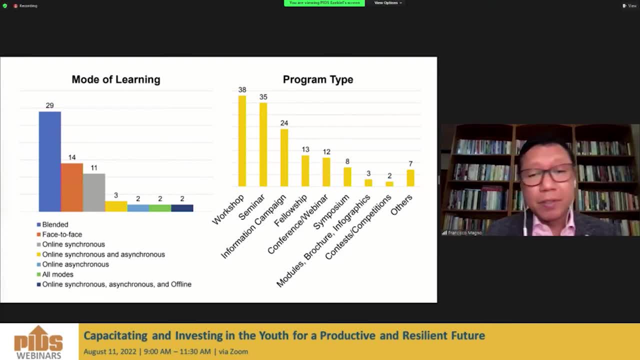 Of course, for NGOs, especially in those in the local communities. they also do face to face In terms of the Yesterday program. if you're all using or following health protocols in terms of program type, you can see on the right side. so, workshops and seminars: information. 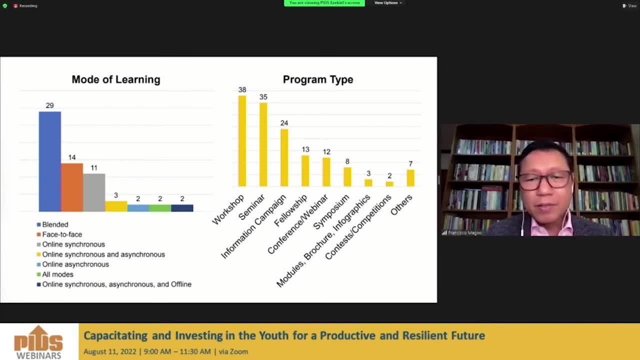 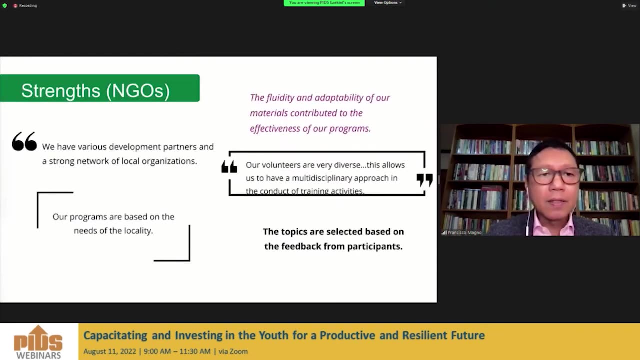 campaigns: Okay, so those are the types of civic education that is rolled out, Usual mainly one to two day workshop or seminar. next slide: Okay, We just have this. Quotes and comments- Okay. Next slide: Okay, from the NGO Key Informants, we have various development partners and a strong network of 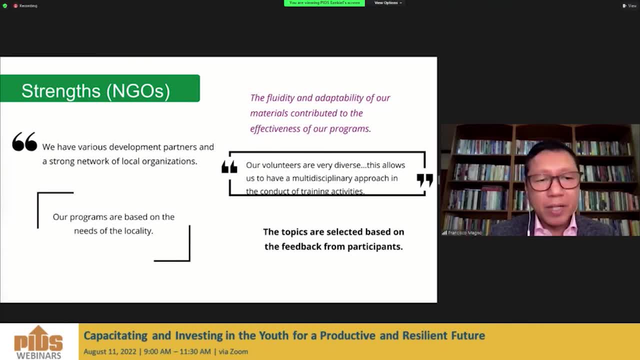 local organizations And our programs are based on the needs of the locality. You can see on the right side of this screen our volunteers are very diverse. This allows us to have a multidisciplinary approach in the conduct of training activities, And the topics are selected. 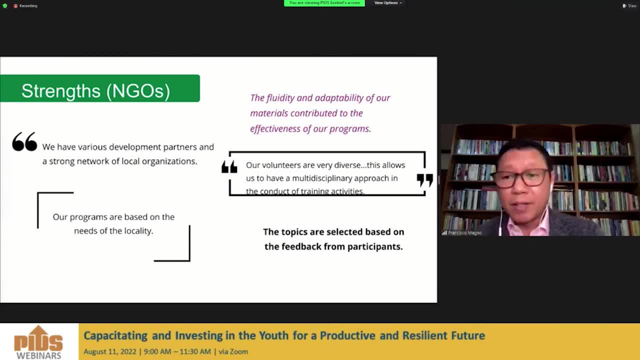 based on the feedback from participants. As you know, it's very demand-driven: the needs of different sectors, different communities. As you can see, the fluidity and adaptability of our materials contributed to the effectiveness of our programs. Next slide: 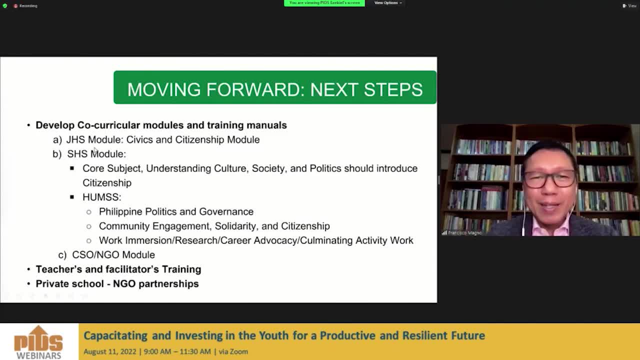 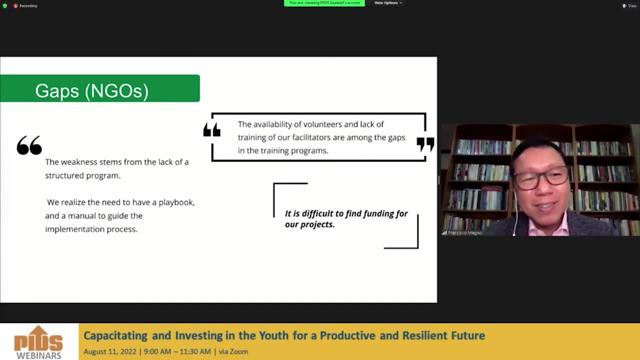 On the gaps. Okay, I think I'm almost done. Okay, the last slide is actually the previous one. The weakness: this stems from the lack of a structured program and we realized the need to have a playbook and the manual to guide the implementation process. 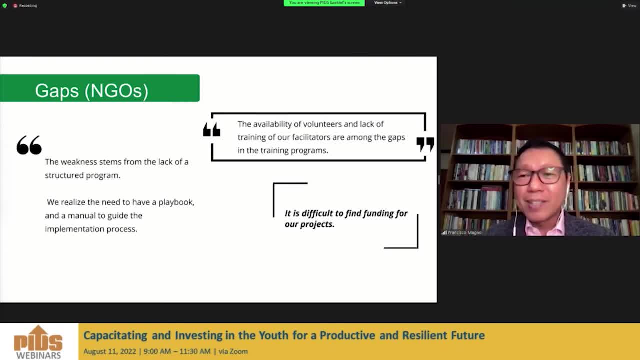 So normally they don't have modules, except for some groups. so what they have are conference programs, workshop programs, and I know this because we also do this kind of training And, yeah, it's difficult to find funding for our projects because 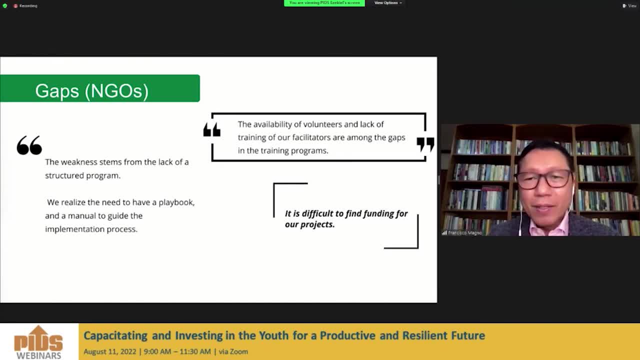 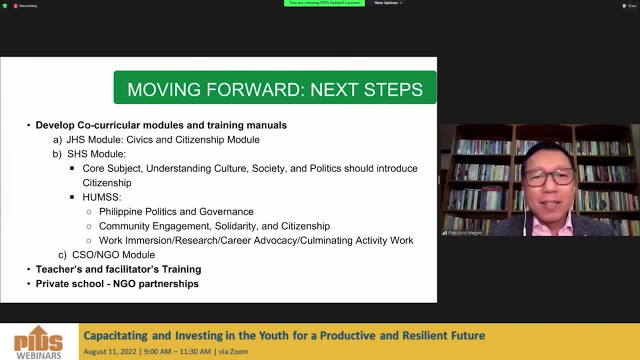 these are voluntary efforts. Next slide: Okay, this is my last slide. These are the next steps that we are undertaking in this project, So developing co-curricular modules and training manuals. When we say co-curricular, ano na yan additional na yan, So pwedeng magkaroon ng mga conference or magkaroon ng guest. 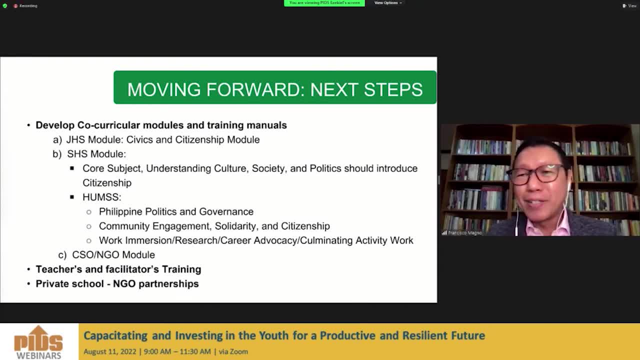 speaker. Iniisip ko nga baka ang dapat na guest speaker yung mga NGOs, kasi marami na silang specific content area, And then teachers and facilitators training and private school and NGO partnerships. So thank you very much. Last slide ko yung thank you.